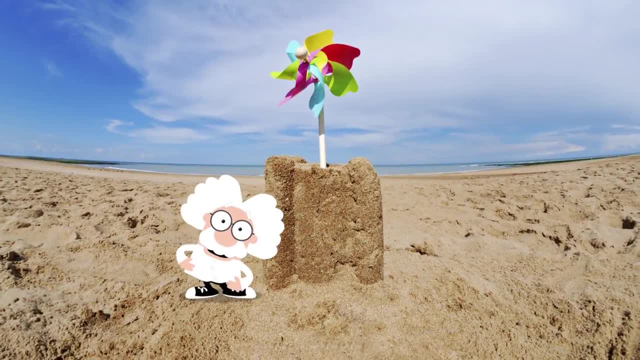 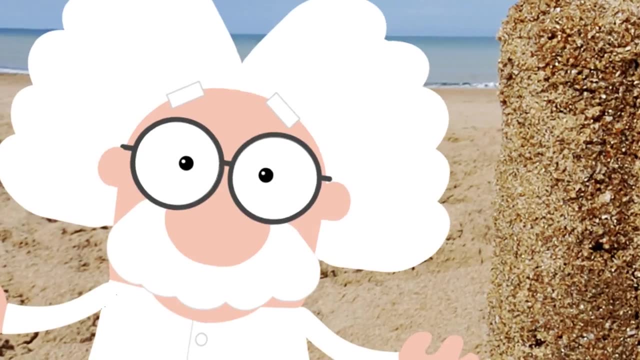 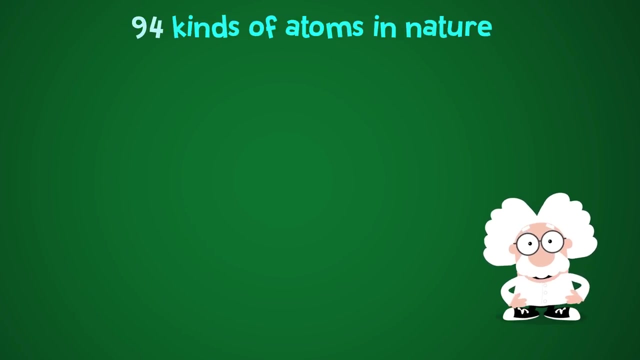 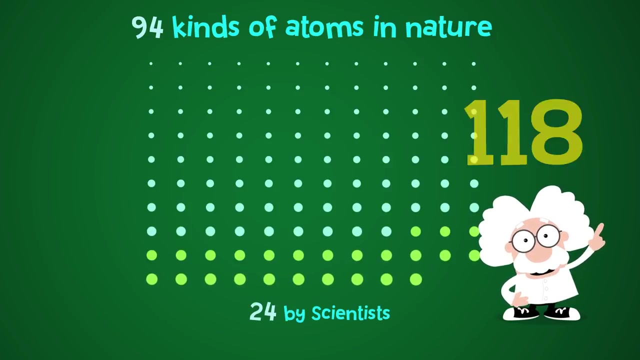 than there probably are grains of sand on the entire beach. Now, that's a lot of very small atoms. Did you know that 94 kinds of atoms make up everything found in nature, And scientists have experimentally created 24 more, which brings the total number up to 118 kinds of atoms? 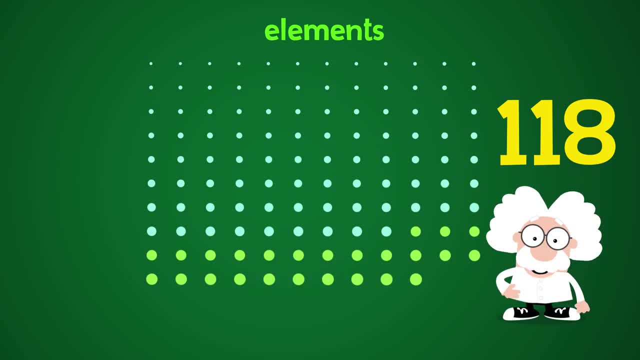 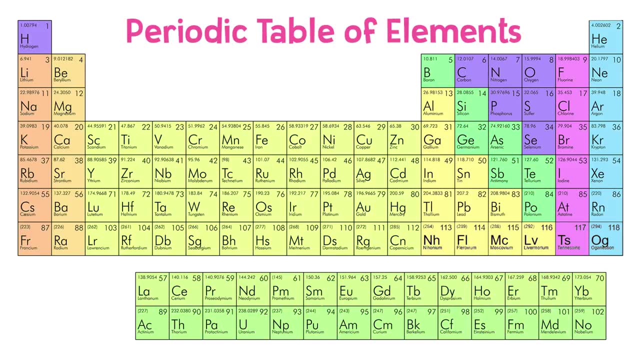 Scientists call them atoms. Scientists call them atoms. Scientists call them atoms. Scientists call each kind of atom an element, And they put them all on this chart called the periodic table of elements. Each element here is special because it looks or acts differently from the other elements. 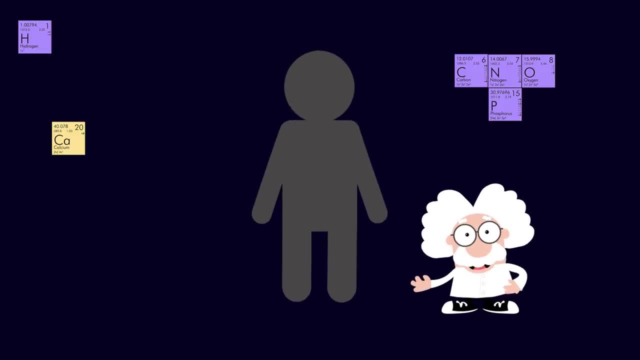 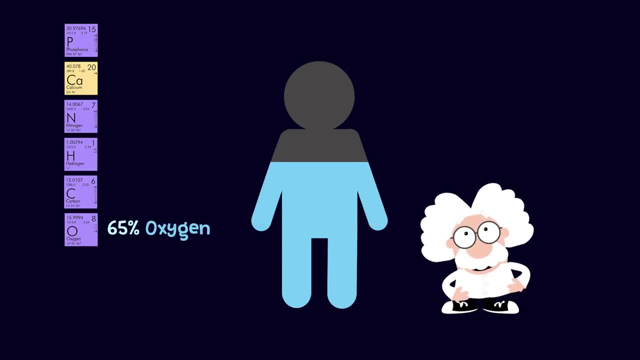 Surprisingly, almost 99% of your body is made up of just six of these elements. You are: 65% oxygen, the stuff we breathe. 18% carbon, the stuff that makes charcoal and diamonds. 10% hydrogen, the stuff that makes the sun shine. 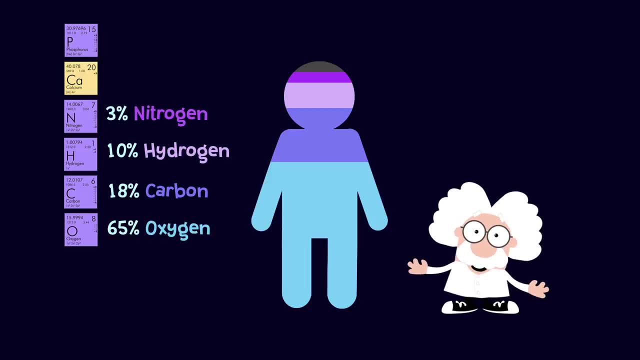 3% nitrogen, which fills most of the Earth's atmosphere, 1.5% calcium, which is good for your bones, And 1% oxygen. 1% phosphorus, a strange glowing element. Now here's the weird part. 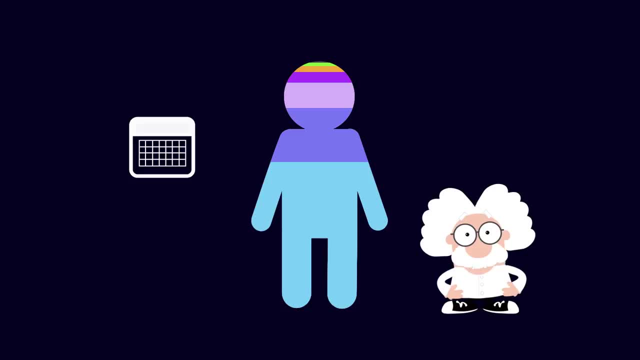 Within one year, almost all of the atoms inside of you will be completely replaced with new ones. How Well we bring atoms into our bodies when we drink, eat and inhale And we lose atoms. We lose atoms when we sweat, exhale or go to the bathroom. 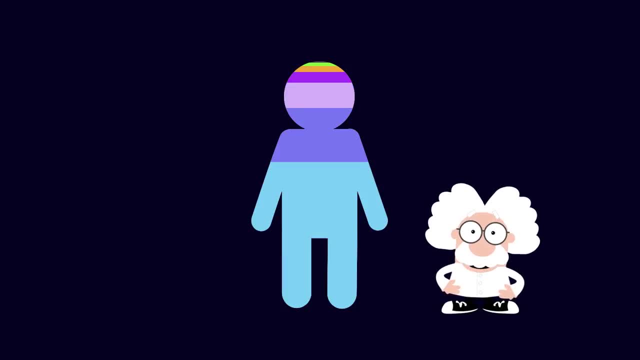 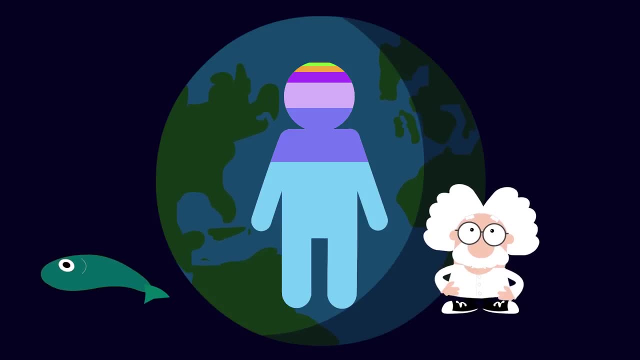 This means you don't just come from the place you were born at, Because your atoms have come from everywhere on the planet: Fish from the sea, Grain from farms, Fruits and vegetables from other countries, And water from everywhere, Everywhere. You are an ever-changing body.